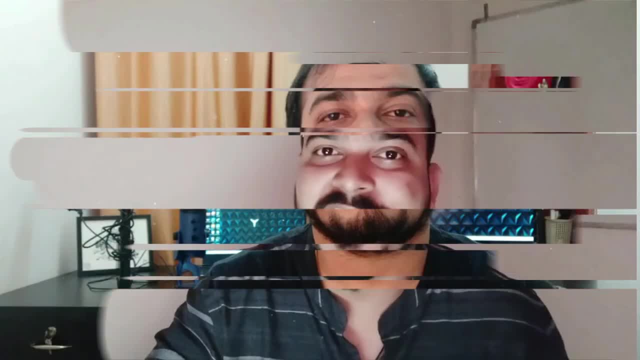 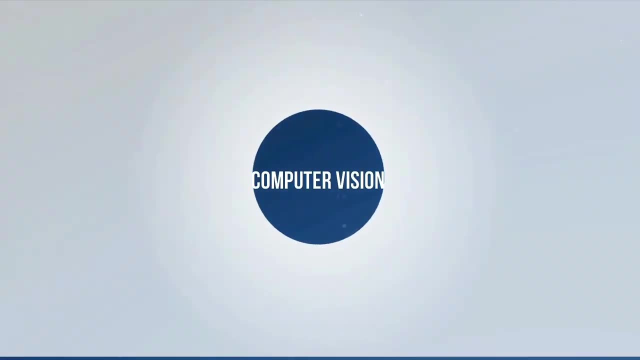 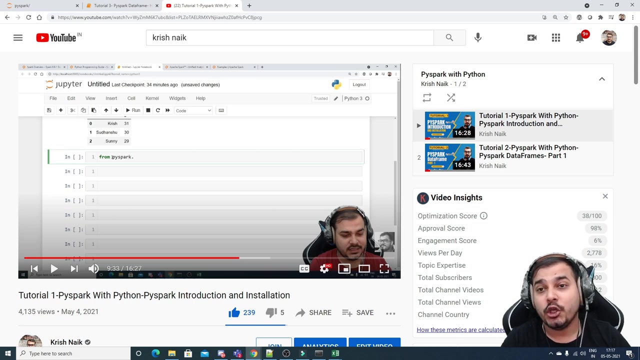 Hello, all my name is Krishnak and welcome to my YouTube channel. So, guys, we will be continuing the PySpark series and I've already uploaded two videos on PySpark. We had actually started the understanding of PySpark data frames. Today we are going to continue and probably this: 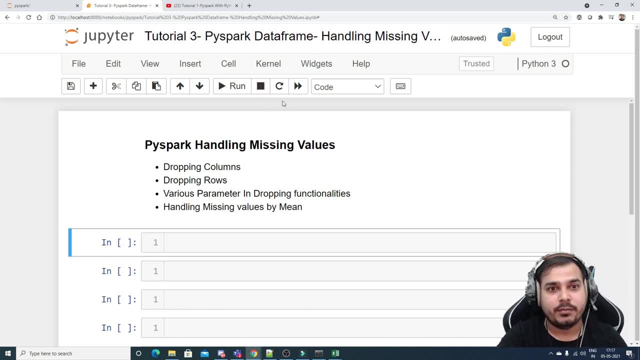 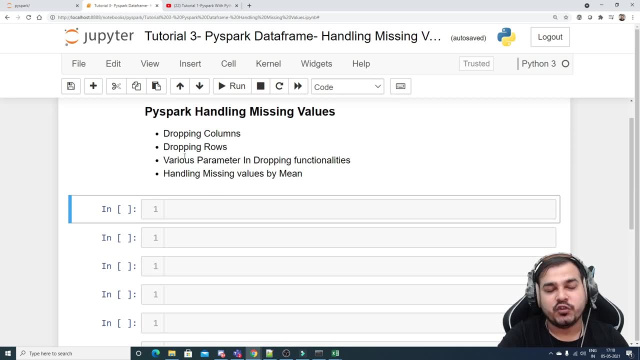 is the tutorial 3, which is the part 3 with respect to data frame operations. In this particular video, we are going to see how we can handle missing values, null values, you know. So, in short, there's many things we'll actually try to do. We'll see how to drop columns, we'll see how 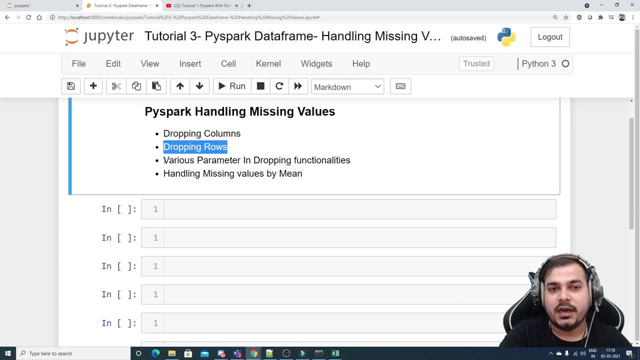 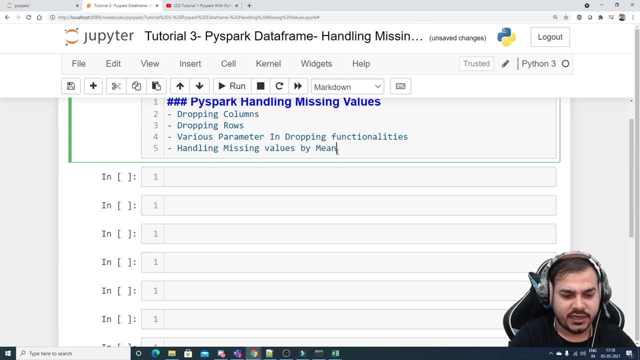 to drop rows, Then we'll see when we are dropping rows, probably based on a null values. we'll try to drop a rows and then we'll try to see what are the various parameters in dropping functionalities and handling missing value by mean, median or mode. Okay, so here I'm just going to write it as: 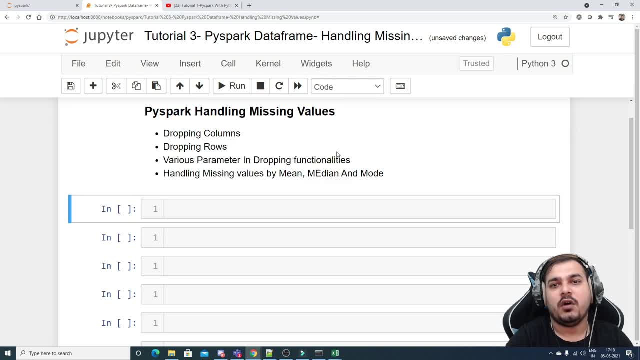 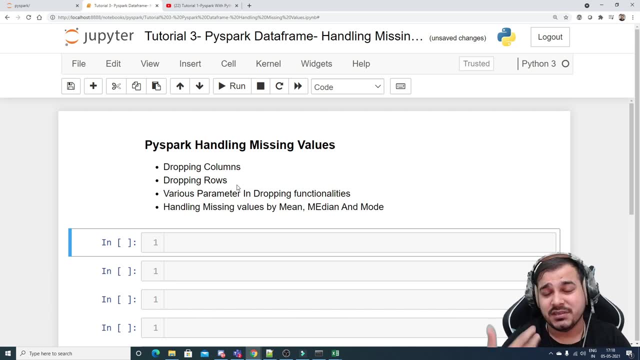 mean median and mode, probably right. So all these things we are actually going to see Again, the main thing is that I really want to show you that how we can handle the missing values. This is pretty much important because in Pandas and all also we try to do this In SQL we have 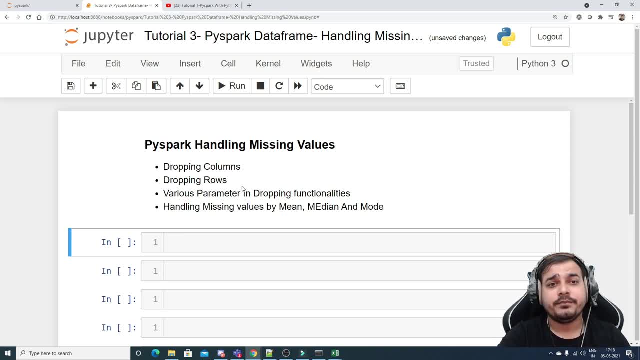 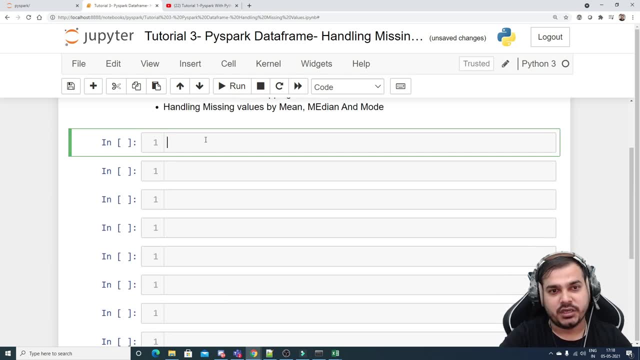 some kind of imputer function. So let's proceed. Whenever we usually start a PySpark, whenever we really need to start a PySpark session, So I hope till now you all are familiar. So I'll write for PySpark dot SQL. I'm going to import Spark session, Okay, and then I'm going to create a variable with 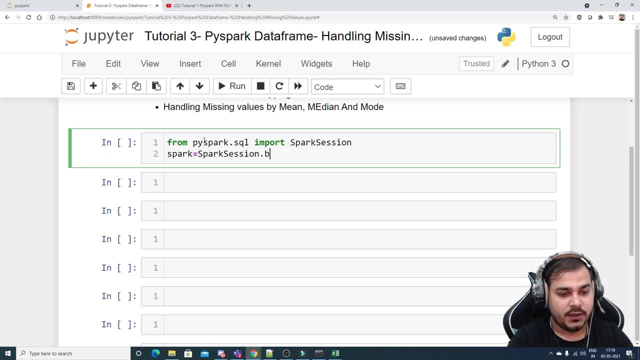 Spark. And then here I'm going to write Spark session dot builder, not app name. Okay, dot app name. Again, let me just keep this app name as practice. Okay, because I'm just practicing things. Then I write get or create and just execute this. 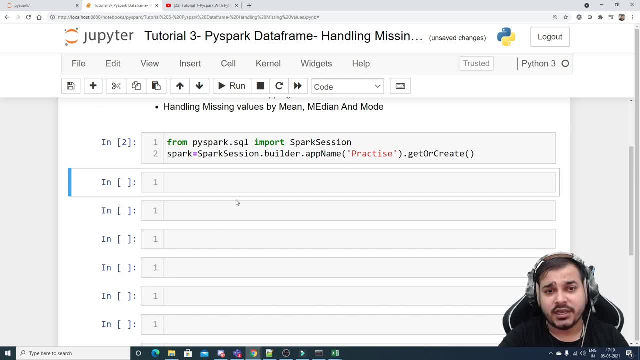 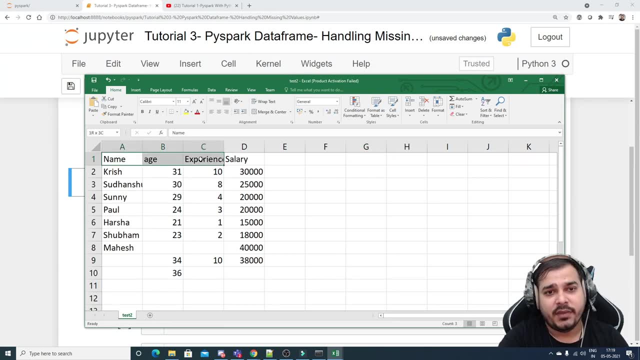 So probably it will take some time to get executed. Yes, it has got executed. fine, Now for this. I've just created a very simple data set which looks like this: I have a column like name, age, experience, salary. So these are all my names, all the candidate names, and probably 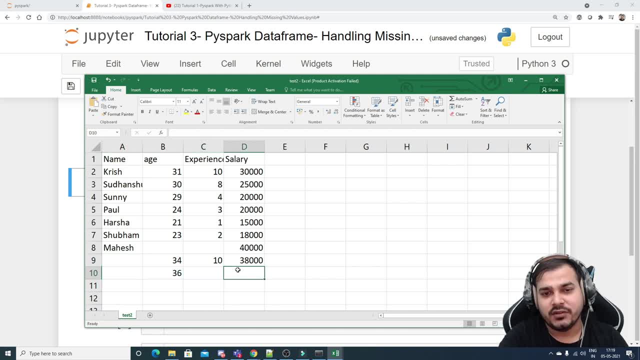 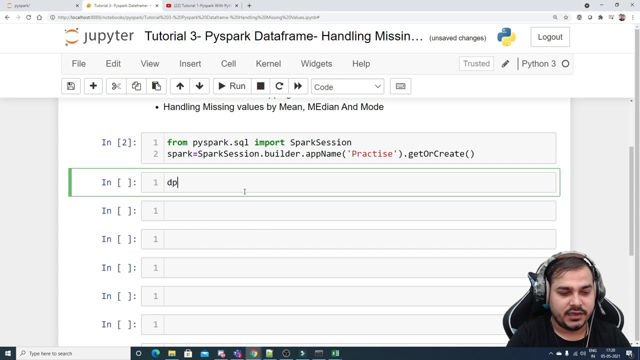 they are some values which are left blank. Here you can see some values are left blank, So we'll hide them. So we can see some values are left blank. So I will take this test And here I'm going to put in the test name and I have the test name is test two dot CSV here And then I'm going. 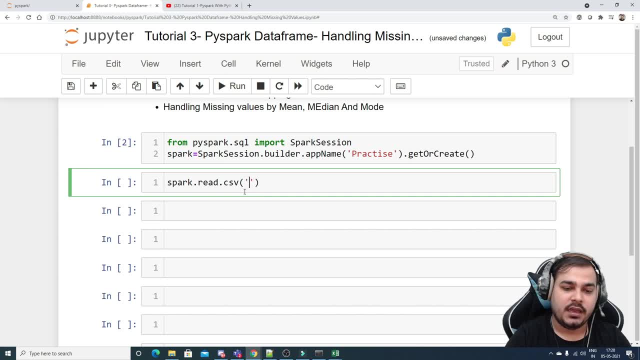 to use header is equal to true. Okay, it will take some time to get computers, So, as I said, I'm going to use header is equal to positive, and probably there is also a file name. So this is going to be the last one I'm going to use. So this is where I'm going to save all these values, Okay. 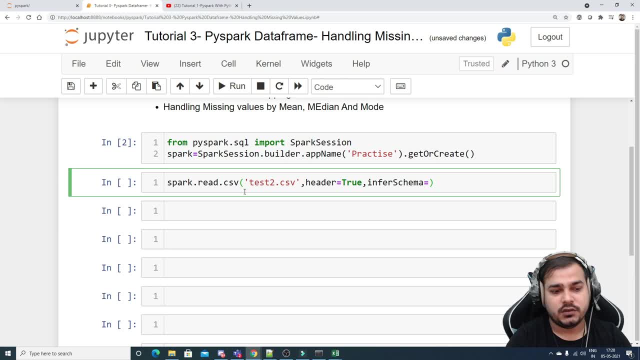 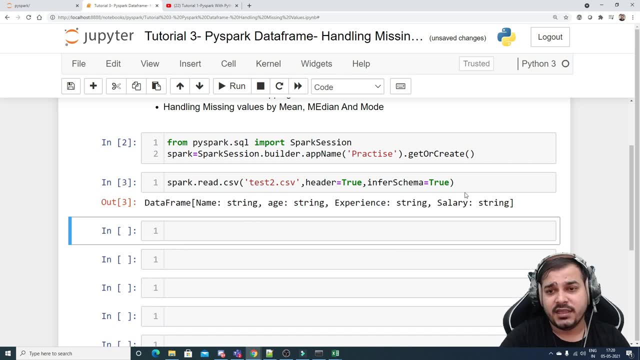 so the first thing I'm going to do is I need to save some of these values, So I'm just going to. there is also inverse schema is equal to true, so that i'll be able to get the data set properly. so probably when i'm reading this, you'll be able to see this is my data frame, that i'm actually 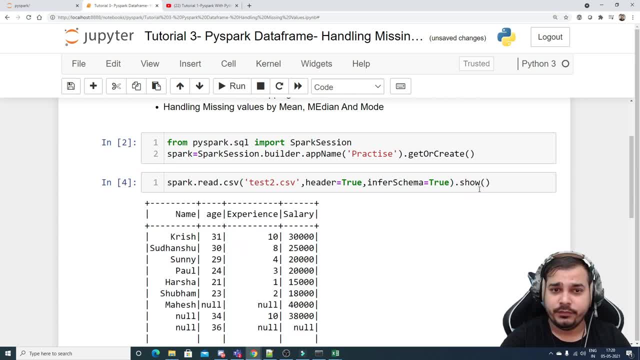 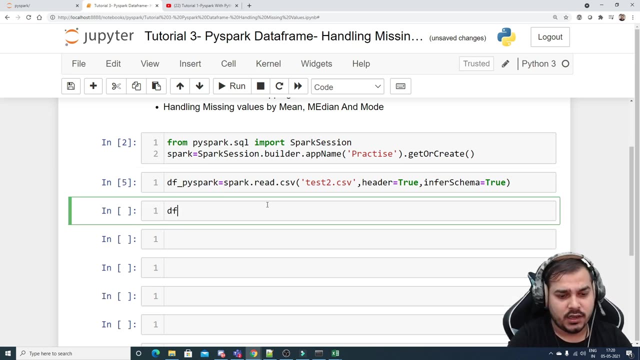 getting. if you want to see the entire data set, this will be like she used dot show and this is your entire data set. here you are having null values and all perfect. so what? let me do one thing. let me just save this in a variable. so i'll write df underscore pi spark. so if i go and now 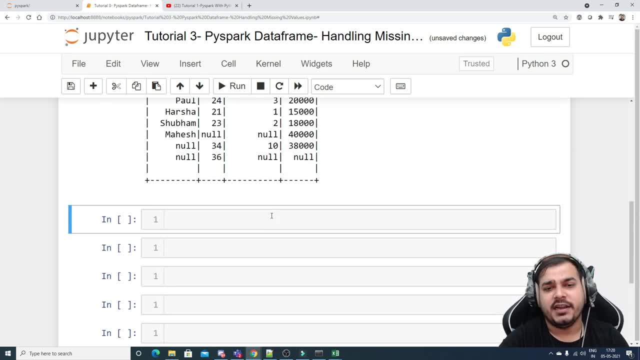 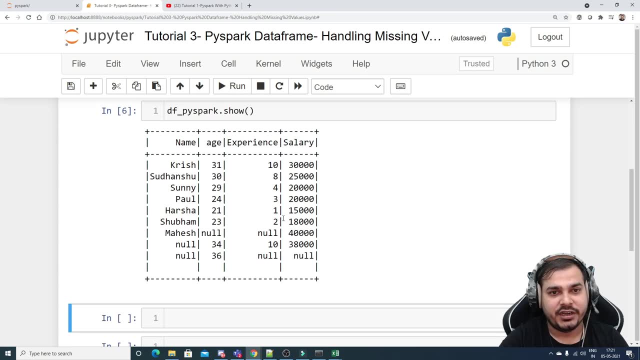 check dot show: this is my entire data set. okay, perfect, uh, we are pretty much good till here. we are working fine. uh, with respect to this, we know we have actually read some kind of data set also. now, uh, probably first let's start. how do we drop the columns? dropping the columns is very, very. 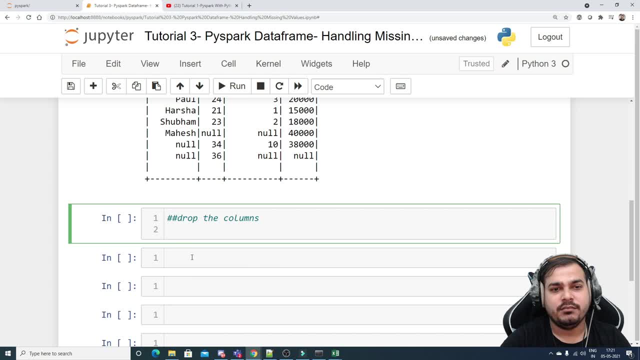 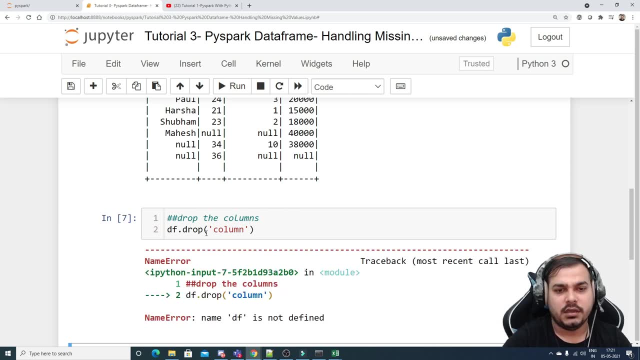 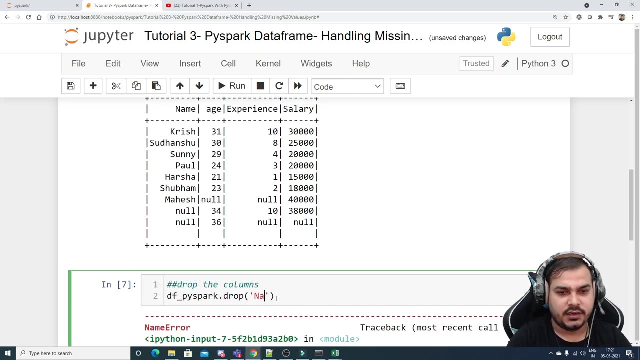 simple guys. suppose i want to drop a name column. then i just use df dot drop and provide my column name like this: right, so column, right, uh, column name. suppose i'll write df dot pi spark and here column name will be name, so let me write it as name. 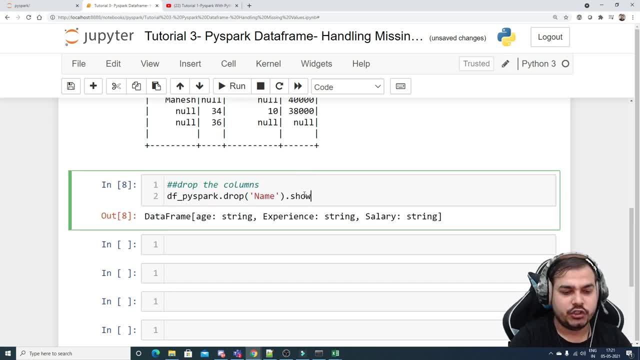 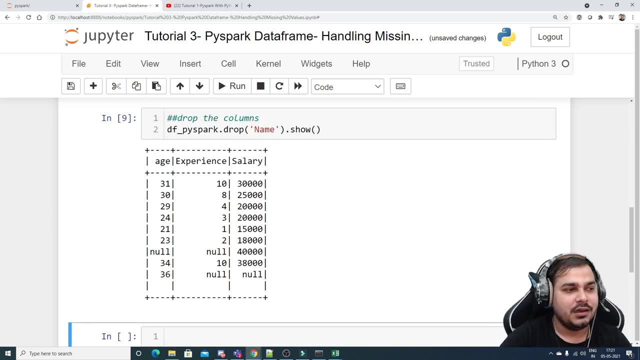 and i can basically go and check out my dot show. then you'll be able to see all the features that are actually present. this is pretty much simple, which i also showed you, probably in the previous session also. okay and uh, this is how it is basically done, basically dropping your uh. 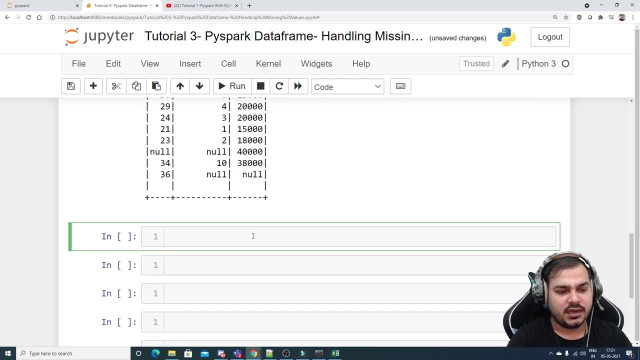 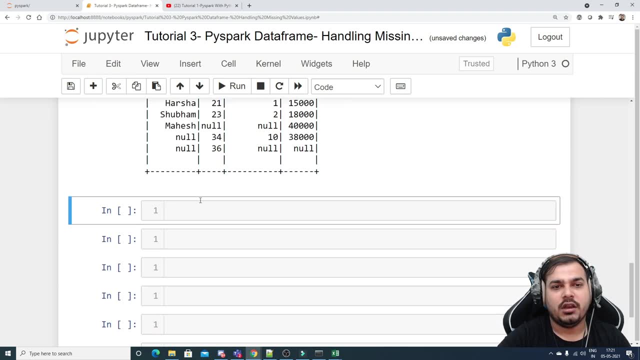 feature or columns, but our main focus is dropping the nan value. so right now let me just write df dot pi spark dot show. so this is my data set, right. uh. now let's see how to drop this specific rows based on the null values. so over here i'll just use df dot pi spark dot na. okay, there's. 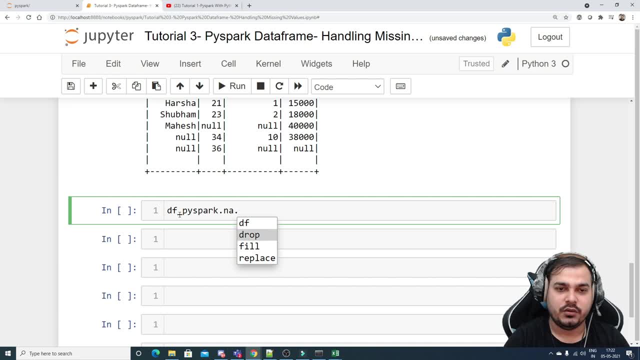 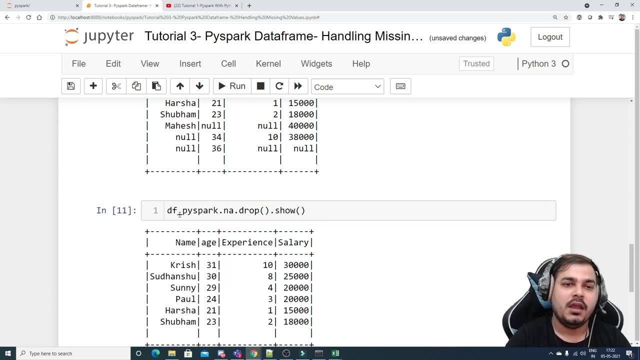 something called as na, and then you have drop, fill and replace. so first of all, i'll start with drop. now, inside this particular drop, always remember, if i don't give anything okay and just execute it here, you'll be able to see wherever there is a null value. 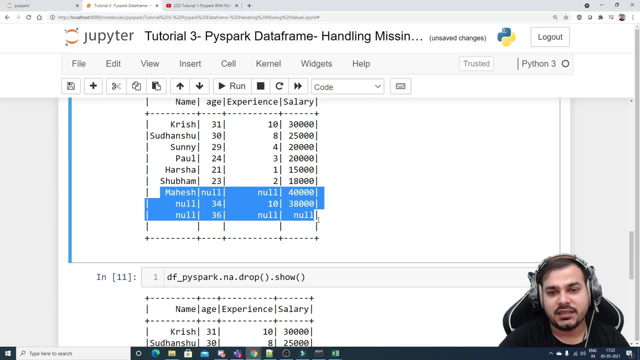 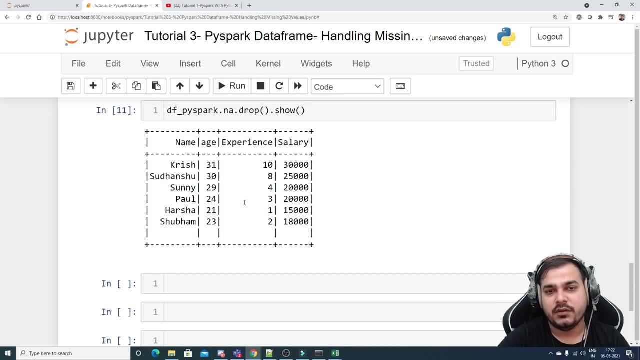 those all rows will get deleted. so here you'll be, seeing that this last three rows are not present, right? so here you can see: till shubham, this particular value is present. remaining all the rows has been removed. perfect, right? so not a problem at all. so here you, in short, what you're. 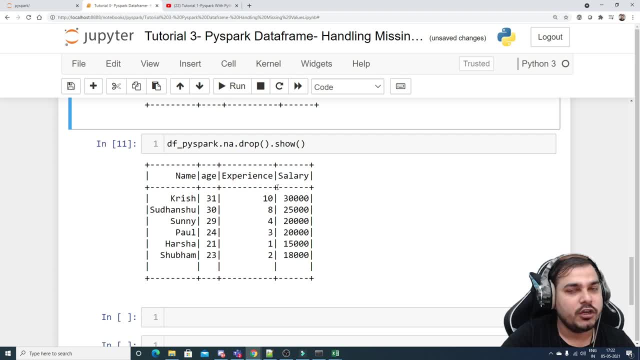 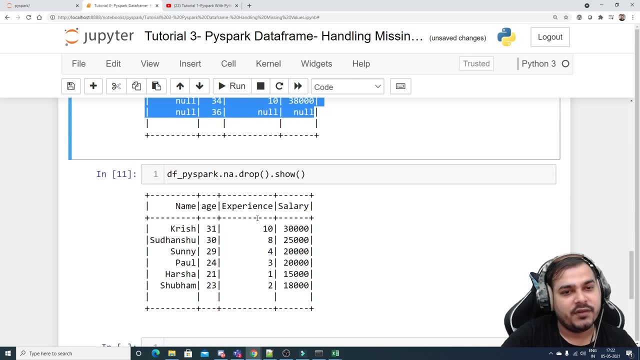 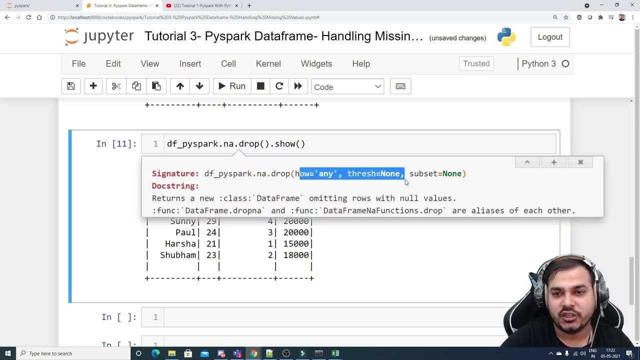 doing is that whenever you use dot na dot drop, it is just going to drop wherever. it is going to drop those rows wherever nan values are actually present or null values are actually present. okay, perfect, this much is fine. if i go and search in the drop, there are two main features: one is how and one is threshold, and then one is subset. so let's try to. 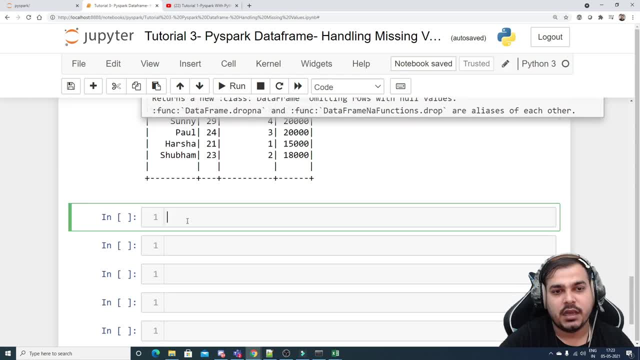 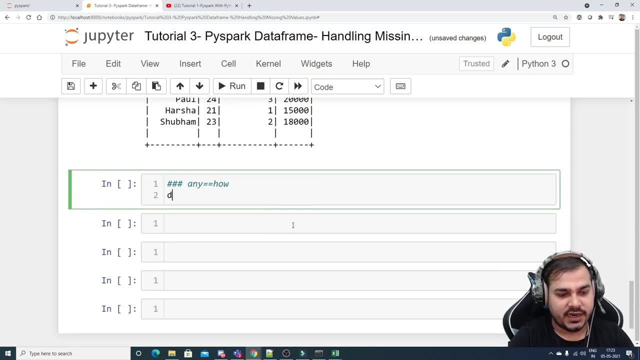 understand this particular features now. first i will start with how. any is equal to how. i'll just write like this: okay, so suppose if i write df, dot, pi, spark, dot, na, dot, drop, and if my how, the how value can have two values: one is any, one is all, okay, one is any, one is all. 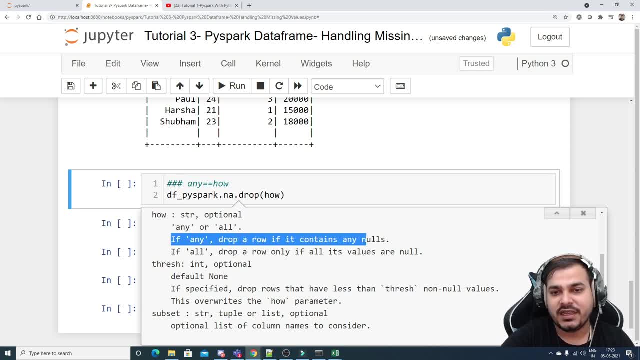 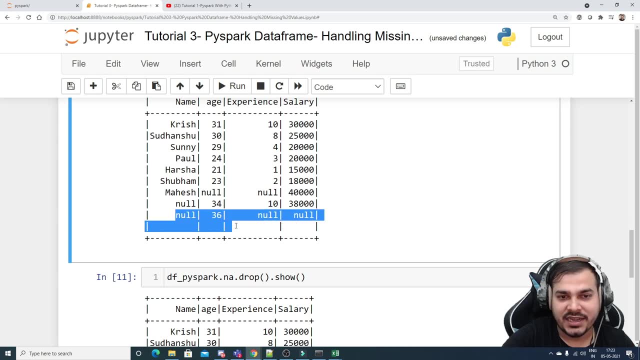 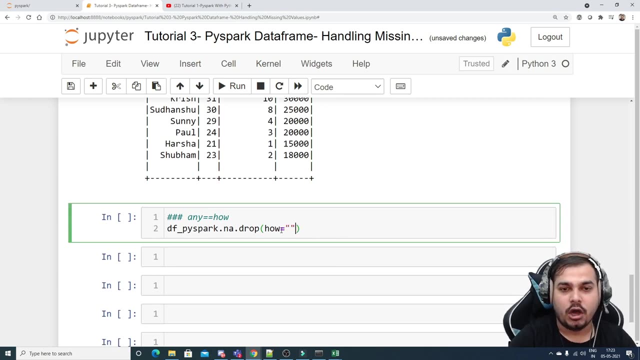 any. if the value selected as any drop or row if it contains any nulls, like even though there is just one null, okay, one null, or there is two nulls, or there is entire nulls, you know, then by default it is going to get dropped. okay, but how is equal to all? when do we use all? that basically means: 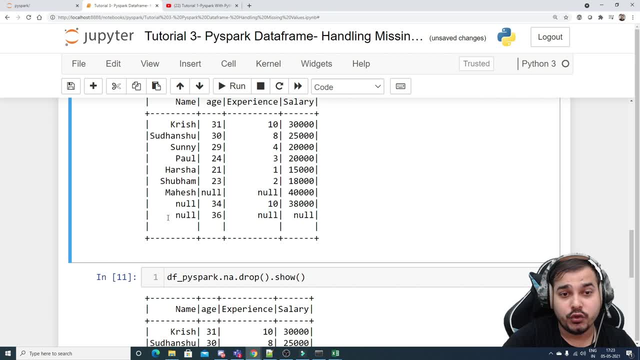 suppose if in your feature you have, suppose, if in your row you have all the values as null- in this case you have 36, one value- this will not get dropped. but if in a record you have all the values and null, then only it will get dropped. okay, so let's see. 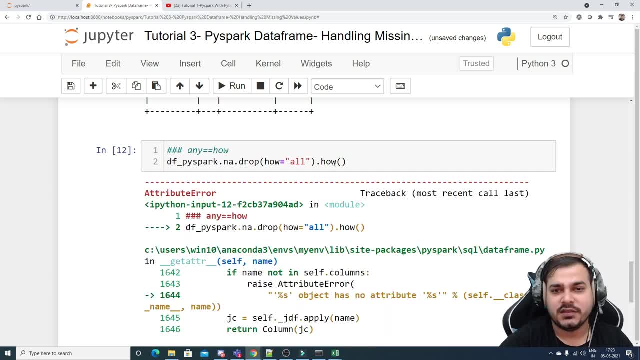 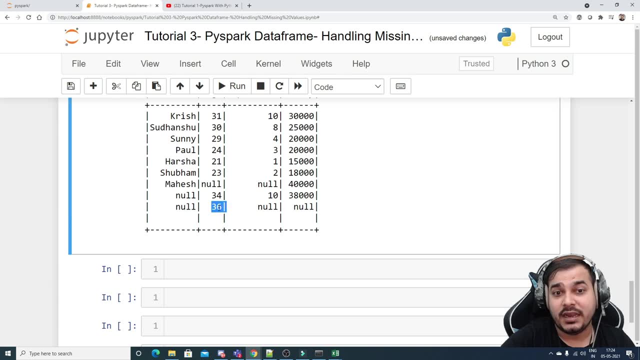 whether this will work or not. definitely it's not going to work because i know all at least one values are at least there. see over here. one values, uh, one, one value. one non-null value is always there, right, if i'm using how is equal to all. it is going to drop those records which is having 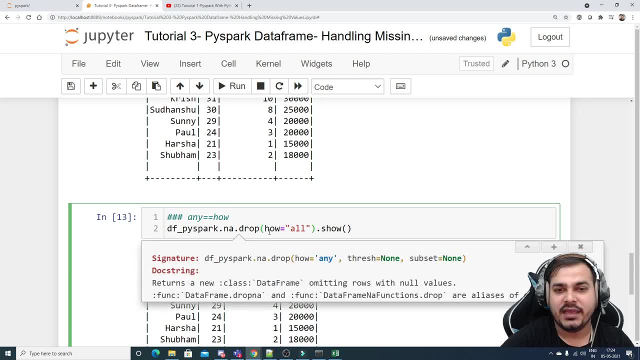 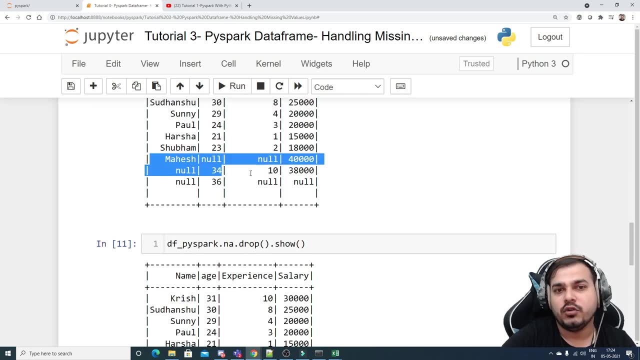 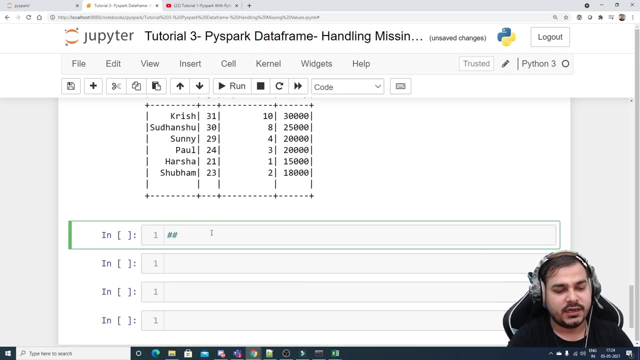 completely null by default. this how value should be having any right, so by default it is any any- basically says that whether there is one null or two null, you are just going to drop it. drop those specific records, right. pretty much simple. this was what how was. now let's go ahead and try to understand. with respect to threshold: 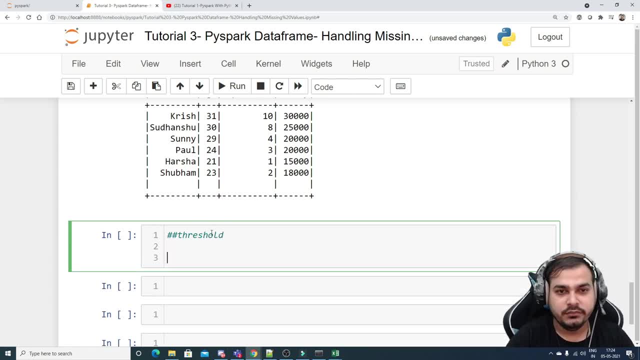 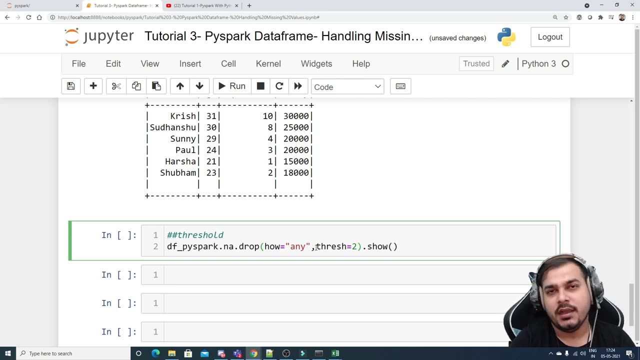 what is this threshold? i'll tell you what is this threshold now. let me just use this. okay, i know how is any, but there is another, one more option called as thresh. now, in thresh, what we do is that, suppose, if i write let's keep the threshold as two, it basically says that: 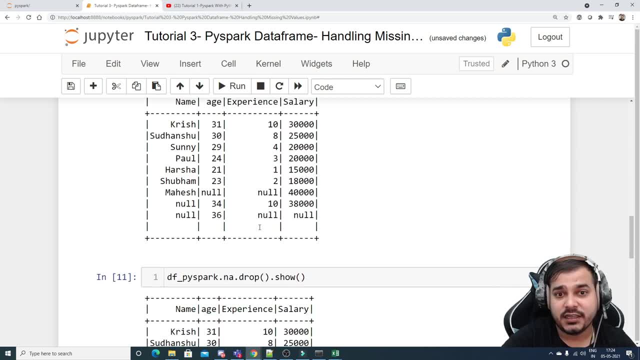 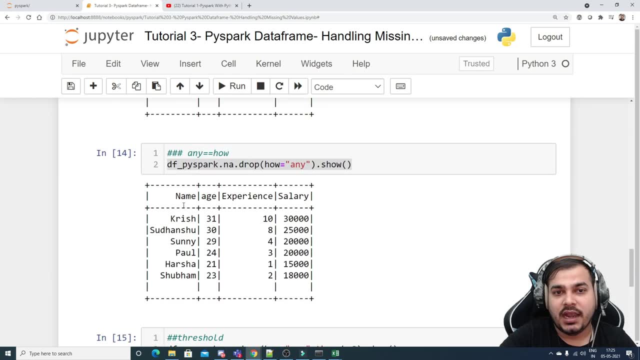 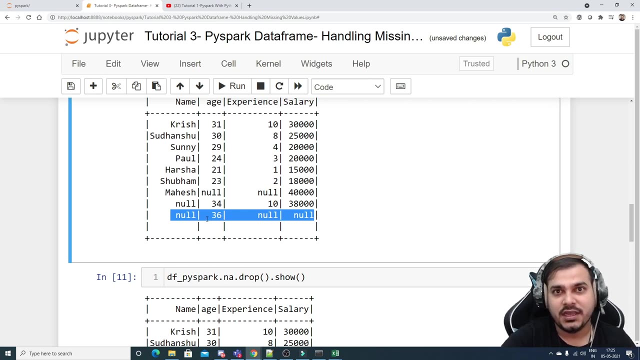 okay, suppose, over here, in this particular case, if the threshold values two, okay, let's, let's First of all execute it. you'll be able to see that the last column has got deleted over here. okay, the sorry last row has got deleted. why it has got deleted? because we have kept the threshold. 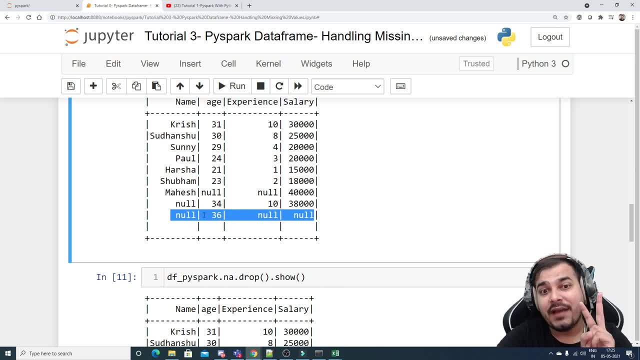 value as two. it says that at least two non null values should be present. okay, at least two non-null values. now, here you have two non-null values: 40,000. okay, here you just have one non-null values. so because of that, it got deleted. suppose, if you had two non-null values over here- see 34 and 10- this is not got deleted, this is same. 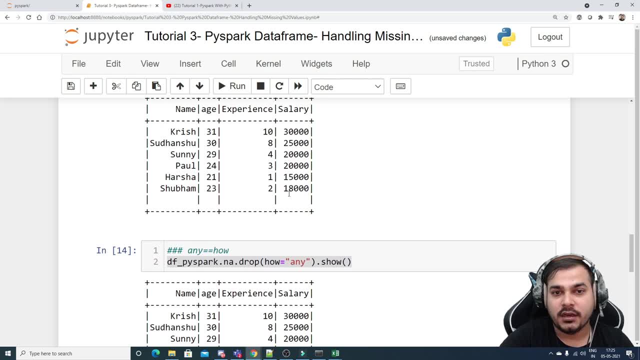 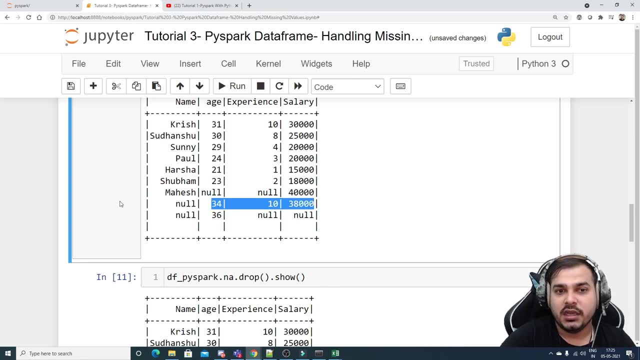 over here: 34, 10, right, 34 10. uh, you have. uh, if i go and show you, 34, 10 over here and 38,000 at least. here you had three non-null values, here you had two non-null values. so here, whenever we, 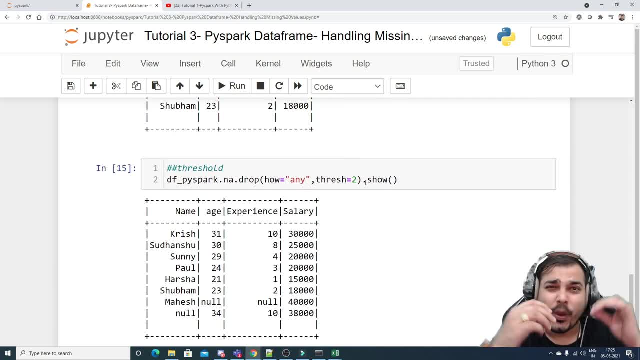 give some threshold value as two. that basically means it will go and check whether in that specific row at least two non-null values are there. if it is there, it is just going to keep that row, otherwise it is just going to delete it. that is what you can know. you can also check out. 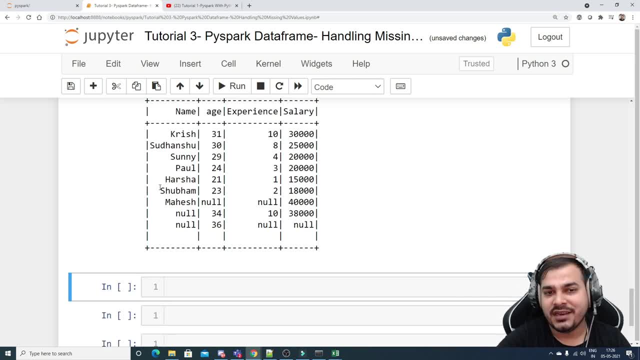 with one. so if i go and see one, then you can see that all this particular rows are there, because it will just go and check. okay, here one non-null values are there. here it is there if i make it as three. okay, let's see what it will come. now, here you can see. at least this is there. 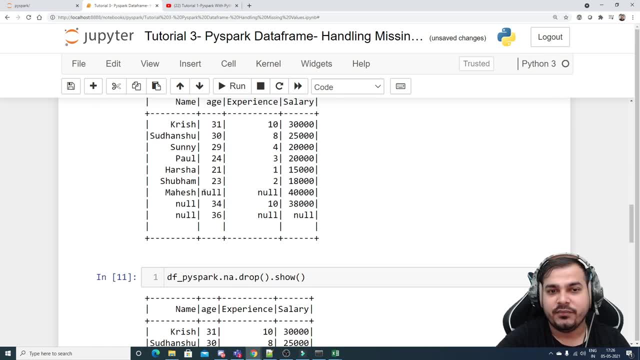 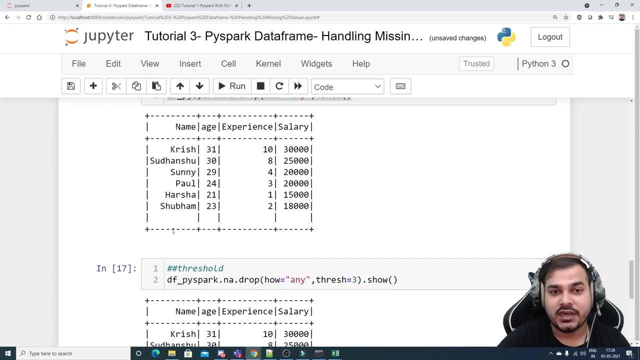 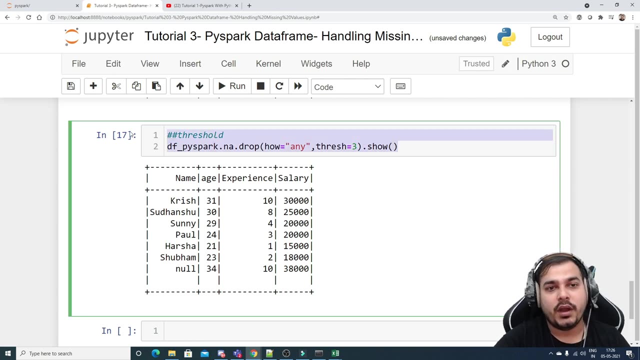 okay, remaining all has been deleted. right, see over here. you had only two non-null values here. also, here you add three. so this is there: 34, 10, 38,000 and null. so here you can see the value. that is the understanding with respect to threshold. now let's go ahead with the another one, which is: 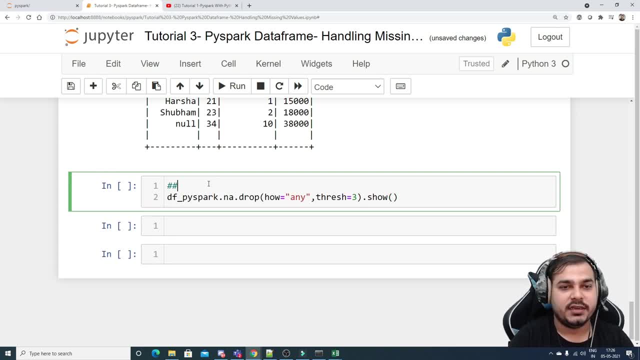 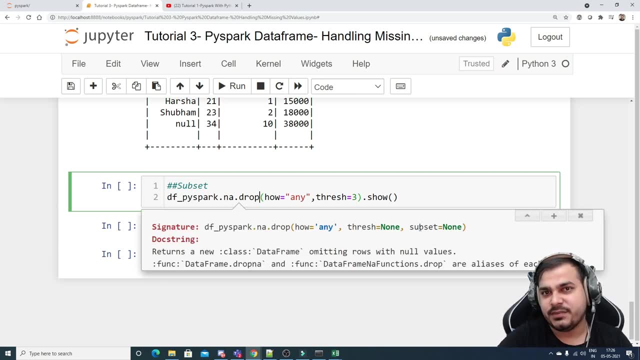 called as subset. so here i'm just going to write it as subset, because this is the third parameter inside my drop feature. and remember these all features are pretty much simple with respect to, if you have worked with pandas, the same thing we are working over here, subset in the subset. we 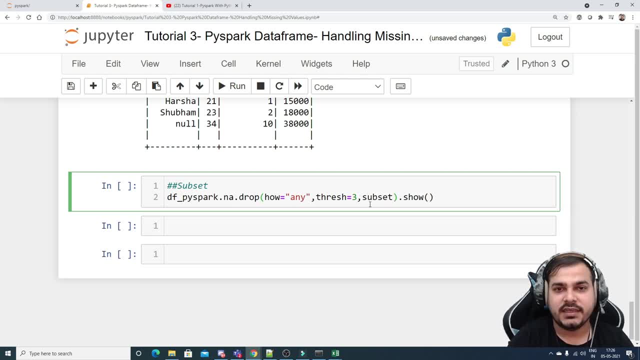 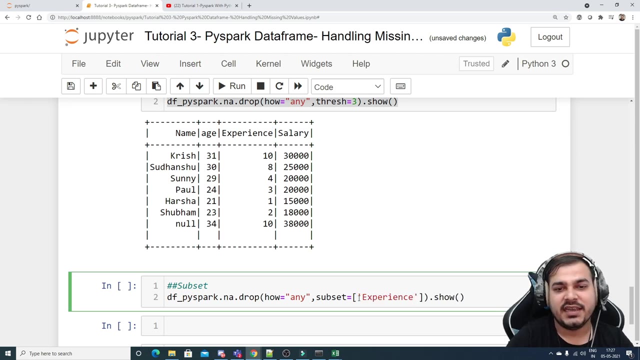 can actually provide. suppose i'll say in the subset: let's remove threshold, i don't want to keep any threshold. let's say i just want to drop nan values only from a specific column, probably only from experience column. then i can basically give it as a subset. so from the experience column. 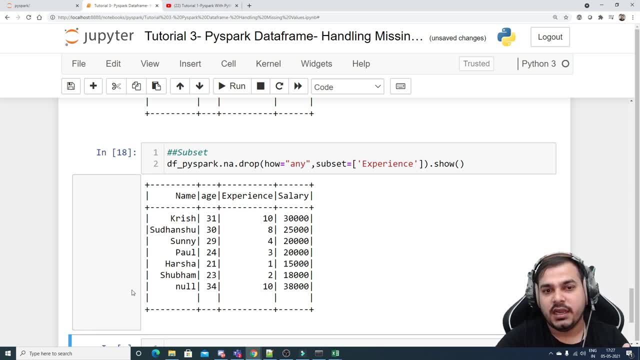 you can see that wherever there was nan values in the records, all those that whole record has been deleted right. so like this you can apply with respect to this- suppose you want to apply it in age- you can also apply this right wherever there was nan values, that whole. 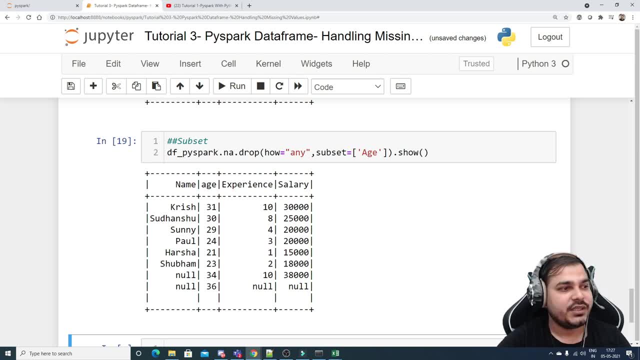 record has got deleted in the age column also, so this is with respect to subset. so i hope you are getting an idea, guys. this is pretty much good because the same thing we are trying to do right, we are actually trying to apply whatever things we actually did in pandas, and this is very, very 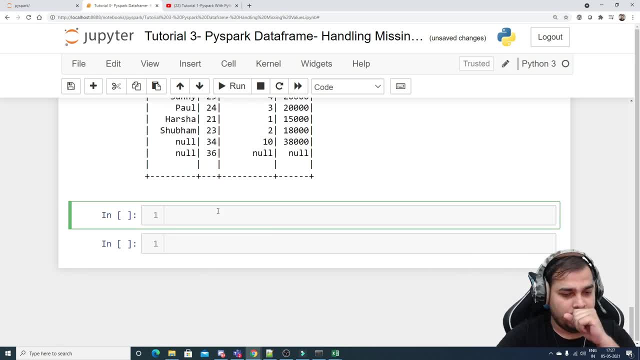 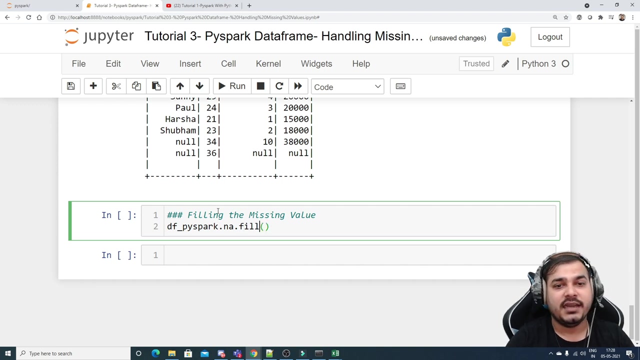 handy when you are working with missing data. okay, let's go with the next uh thing. now let's go and fill the missing value. filling the missing value now. in order to fill the missing value again, i'll be using df by spot dot, fill, dot. okay, sorry, na dot fill, okay. and inside this, this fill will take two parameters. one is value. 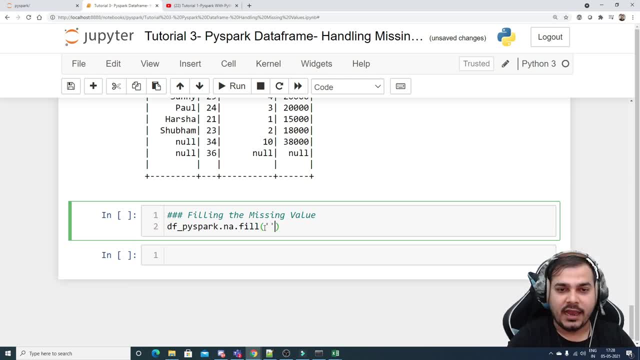 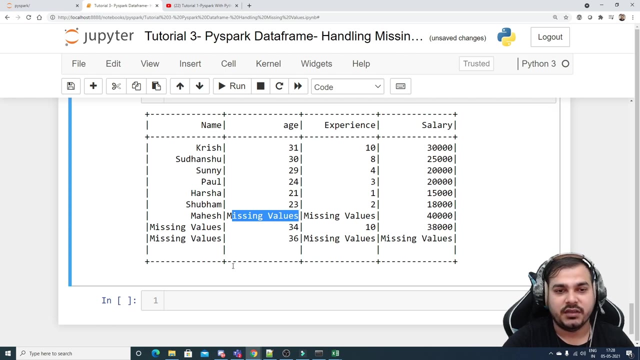 and the one is subset. okay, now suppose if i go and give value like this, suppose i say missing value, and if i go and write dot, then what it is going to do, wherever there is a nan value, it is just going to replace with missing values. so here you can see, here the null value is there. so missing value, missing value, missing. 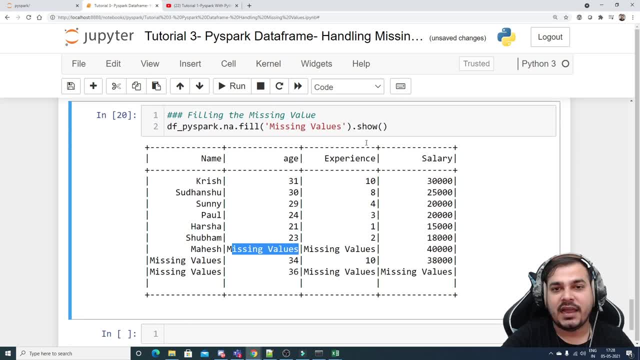 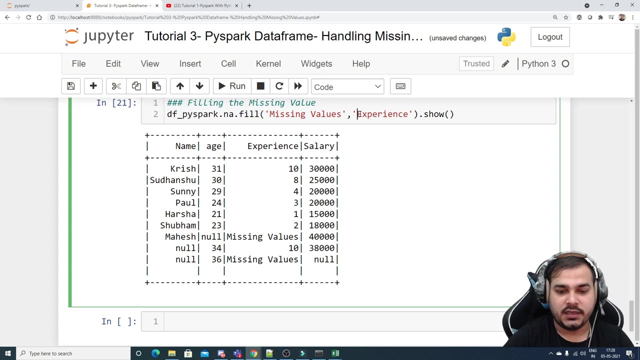 value. suppose if you really want to perform this missing value handling in only a specific column, then you can basically write your column name also like this. so this will be my subset. okay, i can also give multiple records like this. see, i can also give multiple records like experience. 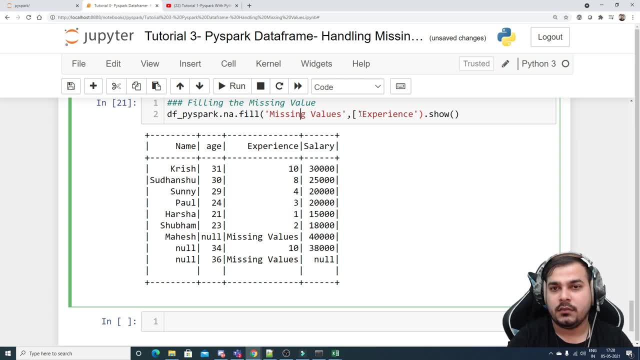 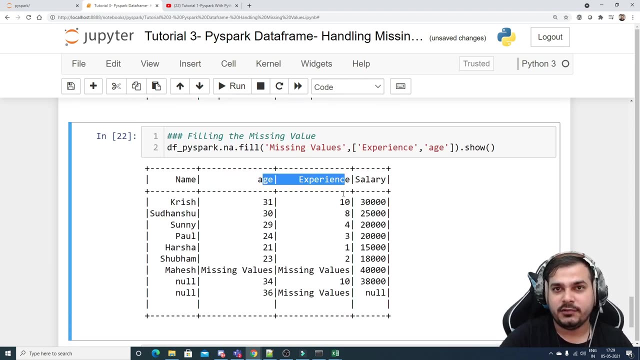 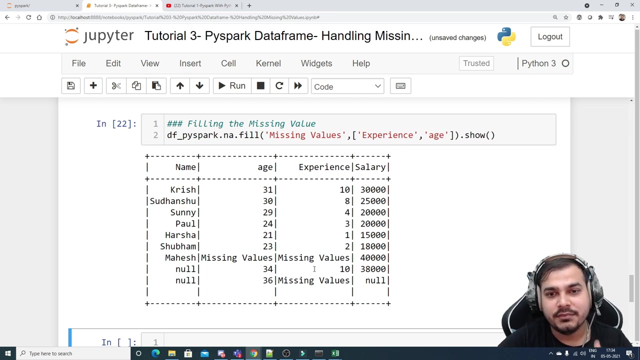 comma, probably age comma, age in call in list, right. when i give like this, then it- this kind of functionality will happen in two columns, right. pretty much simple. so, guys, now next step. what we are going to do is that we are going to take a specific column and probably we are going to handle the missing. 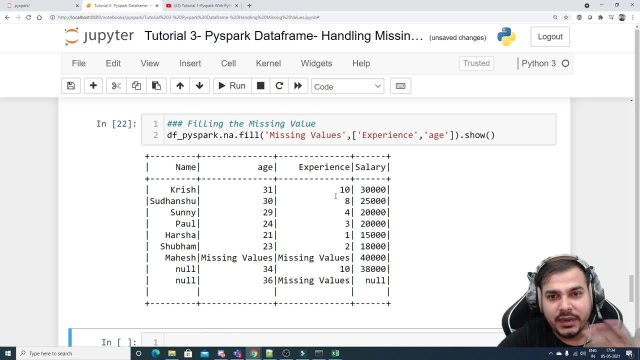 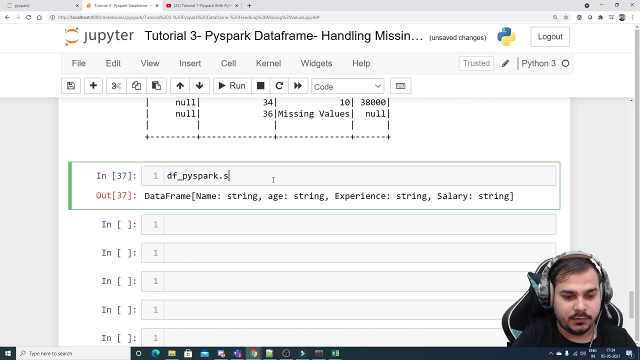 values with the help of mean of that specific column or median of that specific column. so right now we are going to take a specific column and we are going to handle the missing values right now. if i go and check out my dfpy spark here, if i go and see my dot show value, 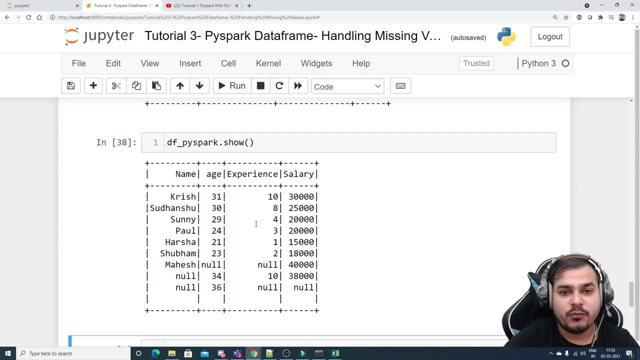 uh, this is my entire data set over here. now what i'm going to do is that i'm going to take this particular experience column and probably replace the null values with the mean of the experience itself. so in order to do this, i'm going to use an imputer function and, guys, if you know about imputer, 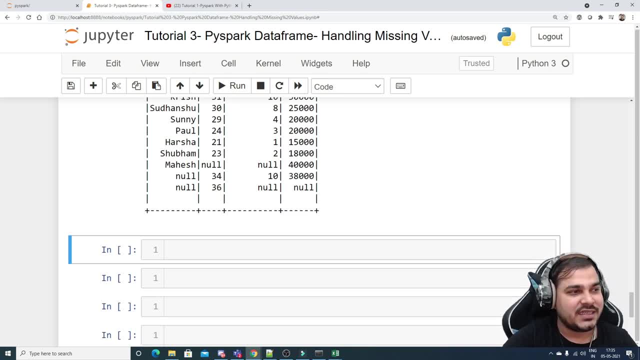 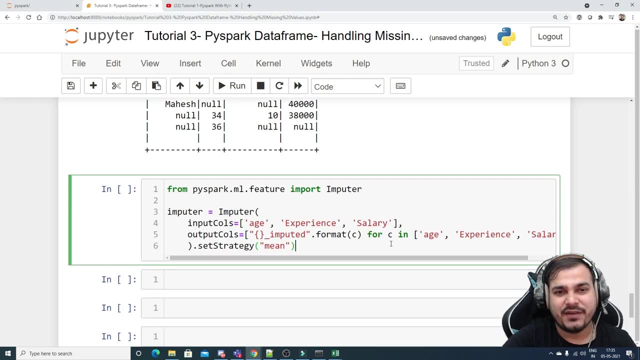 function. um, we basically use that with the help of sk learn also in pi spark also we have an imputer function. so i'm just going to copy and paste the code over here to make it very, very much simple: from py- sparkmlfeature- import- imputer. here i'm just going to give my input columns, that is. 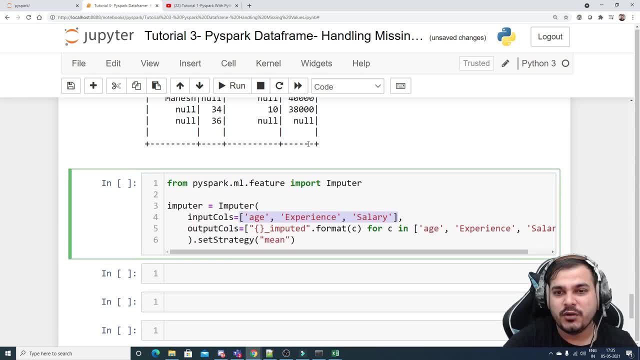 age experience salary. probably i want to apply for every column over here and then i'm just saying that for age experience salary i'm just going to find out this dot formatc output columns and then i'm going to keep the strategy as mean. you can also change the strategy as median mode. and everything. so i'll execute this. this is going to do that by just going to repeat and if this going to work was used, we're going to change the technology. i'm going to just insert the out analyser as mean and change the generating data as is, so that i can understand how measured this actual look is going to change the. 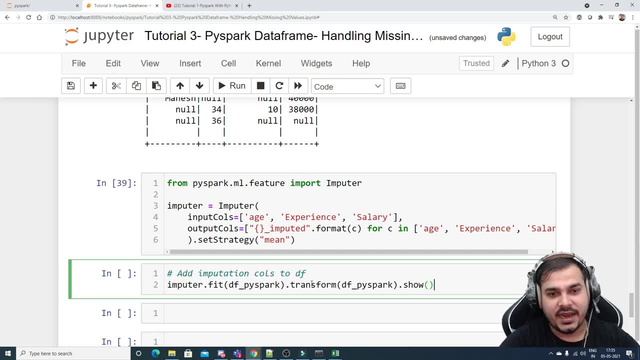 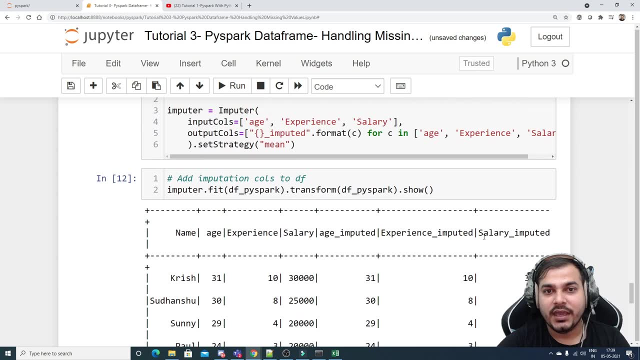 got executed fine, and then we are just going to write fit and transform. so imputed or fit df of pi spark dot transform. so once i execute this, guys, here you'll be able to see that we are going to create multiple columns with underscore imputed as this name. so here you can see age underscore. 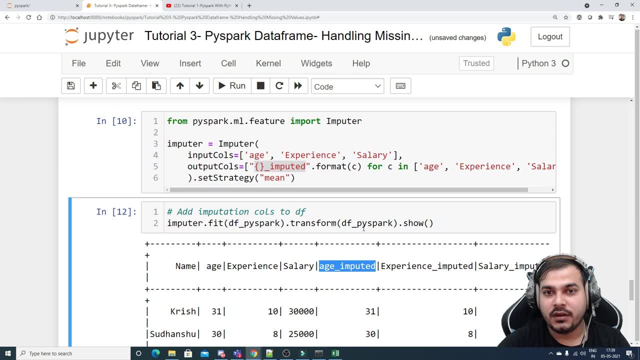 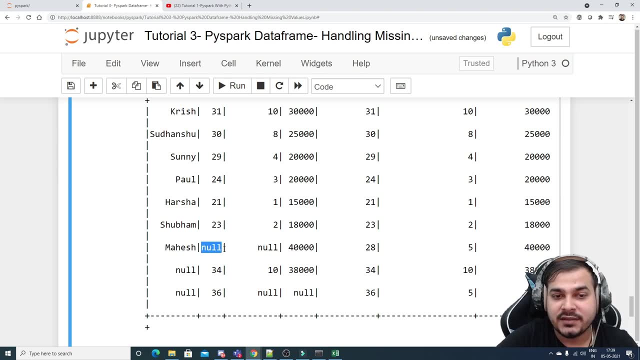 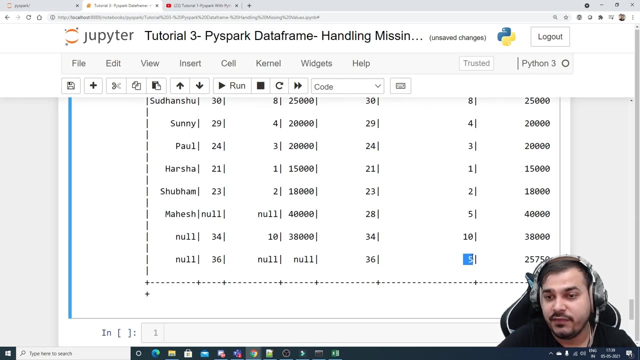 imputed. in short, what we have done. we have tried some kind of uh mean functionality over here. that basically means the null value has been replaced by mean. so uh, over here you can see, this null value is replaced by 28. similarly, this two null value is replaced with 10 and 5. sorry, 5, this is. 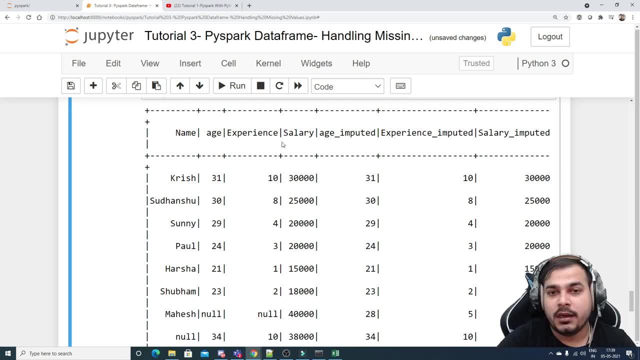 what is the experience imputed column? uh, over here you'll be seeing that wherever there is a null value, it is being replaced by the mean of the experience column, the mean of the age column and mean of the salary column, and this way you'll be able to do it if you really want to go ahead with. 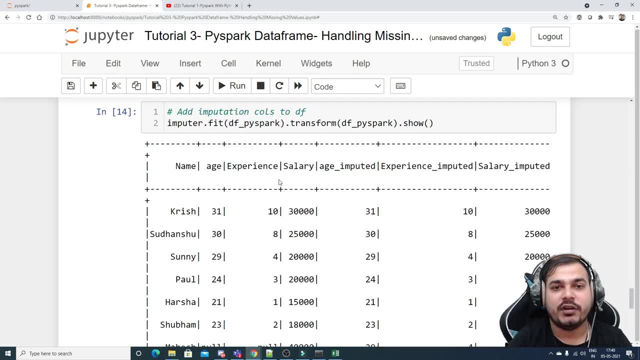 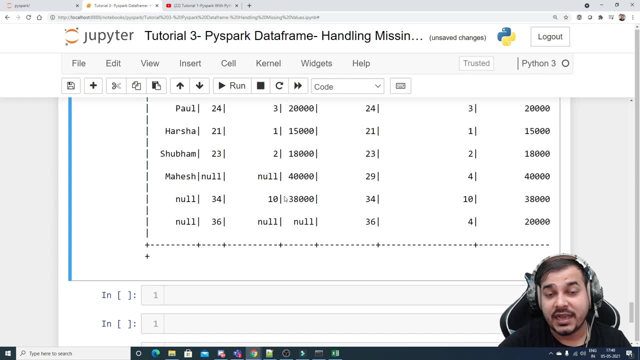 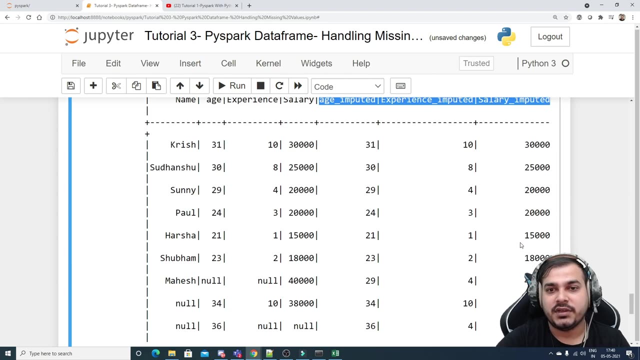 median. just go and change this mean to median and just try to execute it here. now you'll be able to see the median value. and here is your initial null columns which have- sorry, here are the columns which has null values and here are all the columns which has basically the imputed values, right with respect to mean. 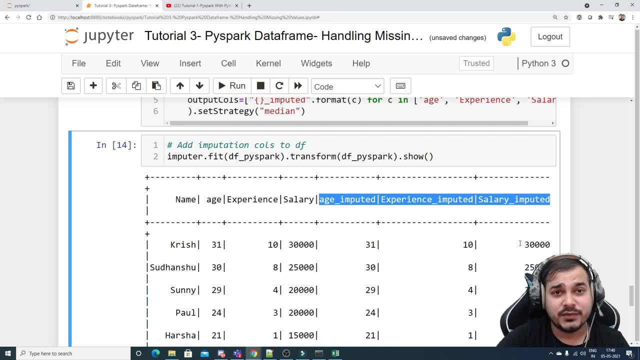 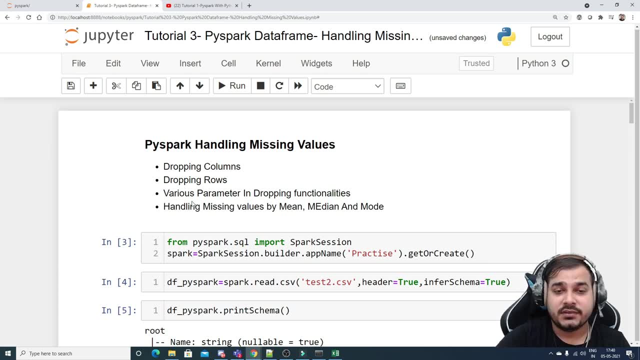 median, so i hope you like this particular video, guys. uh, this was with respect to tutorial 3, and in this video we have tried to see how to drop columns, how to drop rows, how to uh check out various parameters with respect to dropping functionalities and handling missing. 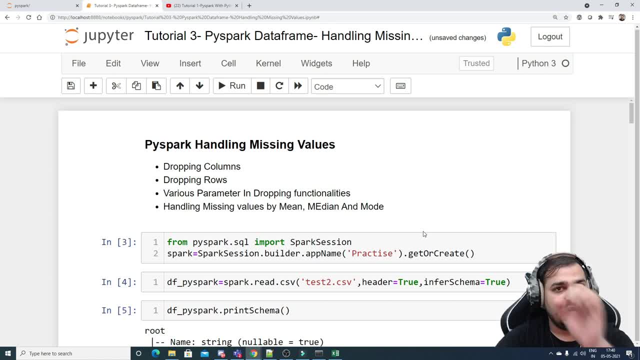 values by mean, median and mode. you can also try out mode. it is up to you and you can definitely just try it out and try to see whether you are able to do it or not. so i hope you like this particular video. please do subscribe to the channel if you're not already subscribed. 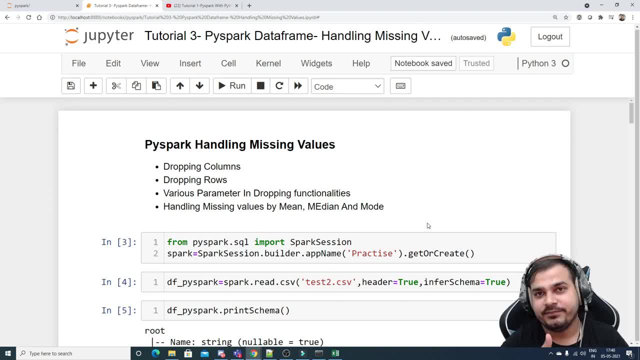 i'll see you all in the next video. have a great day and thank you and bye.